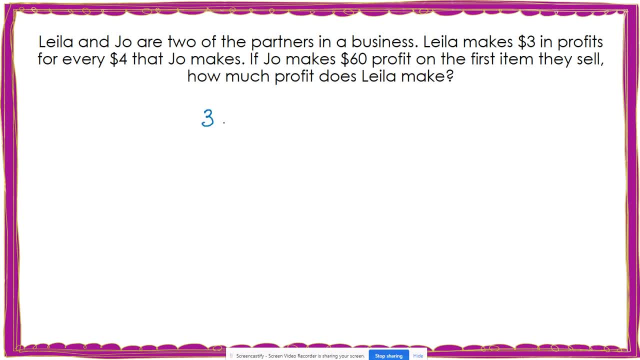 makes three dollars profit. so we can say Leila makes three dollars for every four dollars that Joe makes. So the proportion that would represent this is three dollars to four dollars, and three dollars represents the profit for Leila, four dollars represents the profit for Joe. I can make a proportion by setting this equal to another ratio. 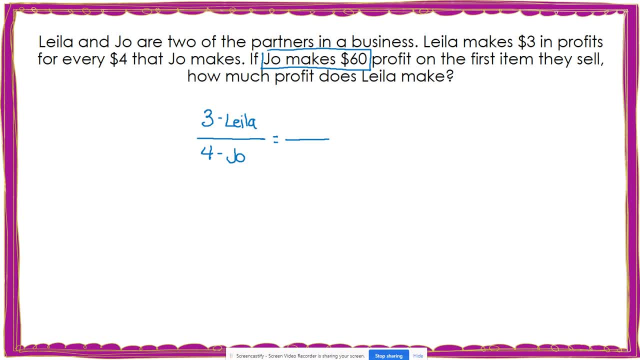 and in this ratio I know that Joe makes a sixty dollar profit. So since Joe is in my denominator on my first ratio, I'm going to put Joe in my denominator for my second ratio. What I don't know is how much profit Leila makes, Since I don't know that value. 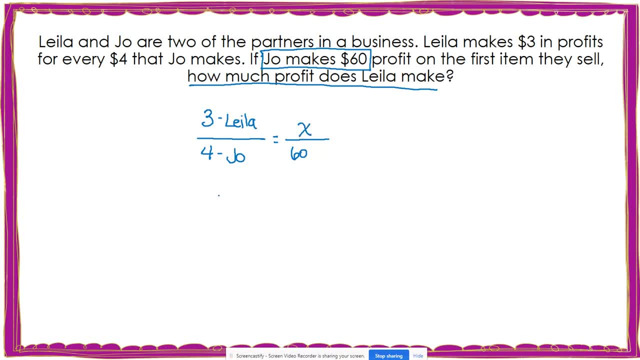 I'm going to use a variable to represent it. Now there are different ways to calculate the ratio to the number of dollars that Joe makes that we can do this previously. you've learned that. i know that if i'm moving from 3 to x, i 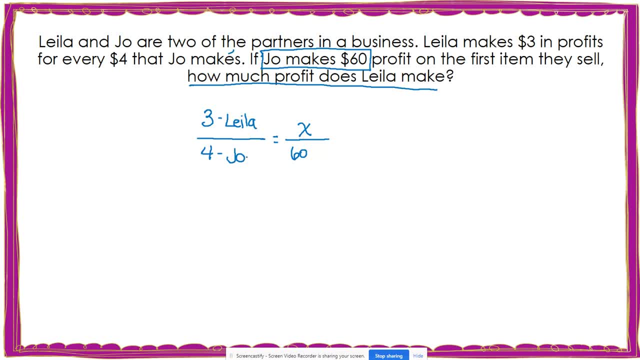 can figure out how i moved from 4 to 60.. i know that to get from 4 to 60, i would multiply 4 times 15 and since this is changing at a proportional rate, i would also multiply 3 times 15 to get x. 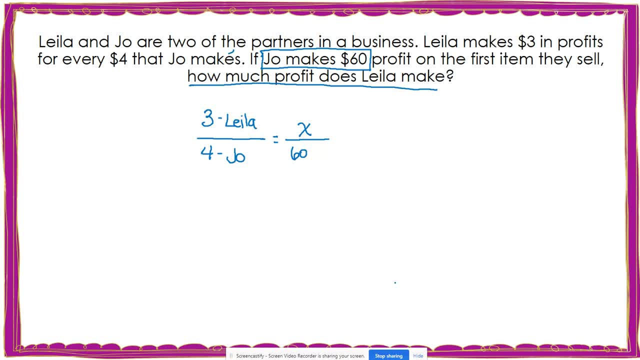 sometimes we have values that aren't that friendly and they are a little bit difficult to do things like that with. so in those cases we can cross, multiply and make an equation. when we cross multiply, we start with the numerator from the first ratio and multiply it by the denominator. 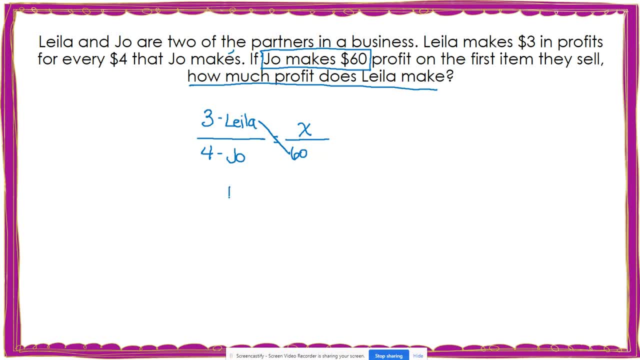 in the second ratio. so we would multiply 3 times 60 to get 180.. then we would write an equal sign. next we would multiply the numerator from the second ratio by the denominator in the first ratio. so x times x, e, the denominator from the second ratio is equal to 6tenteen side punishment. must occurred. using this, it's not a problem. if you got a number in a Lives1 argument, you're able to use this 대표 from an derivative method to calculate x minus 2 times here. then it's excellent when you know the square root of f is required. but you don't have to think aboutBYO, but you have. 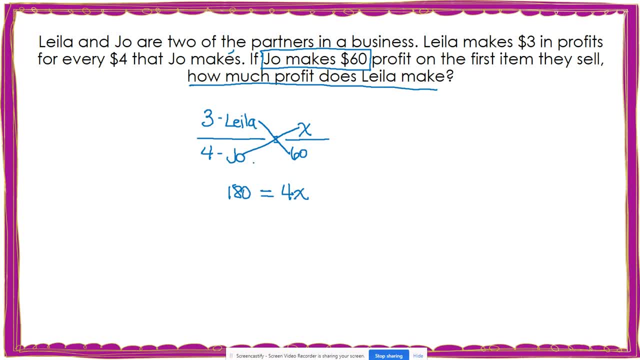 four would give us 4x. now all we would need to do is solve for X using inverse operations. since X is being multiplied by 4, I know that I need to divide by 4 on both sides of my equation. if I divide by 4, 180 divided by 4 will give me 45. 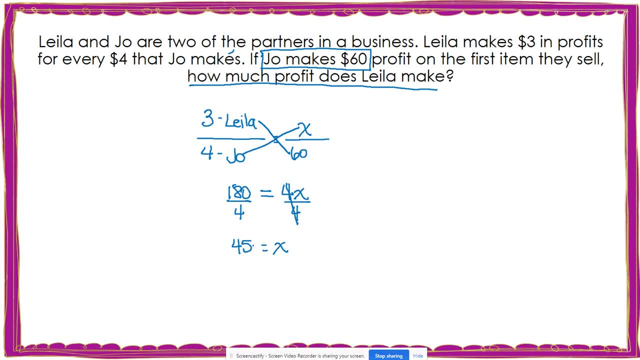 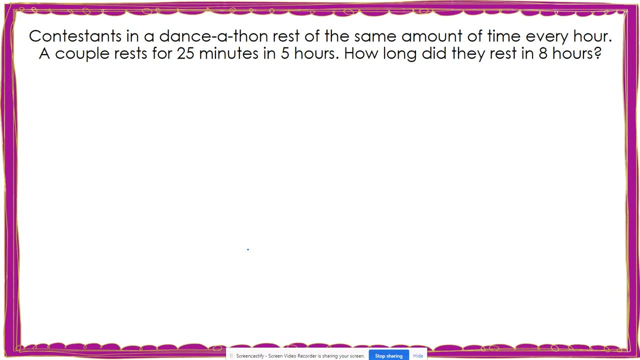 these fours will cancel and leave me with X. this means that if Joe makes a $60 profit, Lila makes a $45 profit. next, I see that contestants in a dance-a-thon rest the same amount of time every hour. a couple rests for 25 minutes in 5 hours. so how long did they? 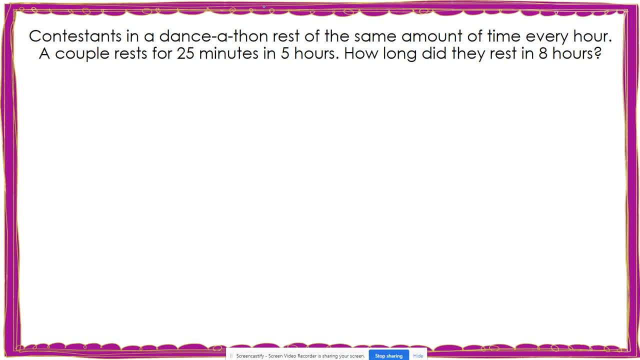 rest in 8 hours. well, the first thing I can do is make my first ratio from my first ratio. I know that the couple rests 25 minutes in 5 hours. well, the first thing I can do is make my first ratio from my first ratio. I know. 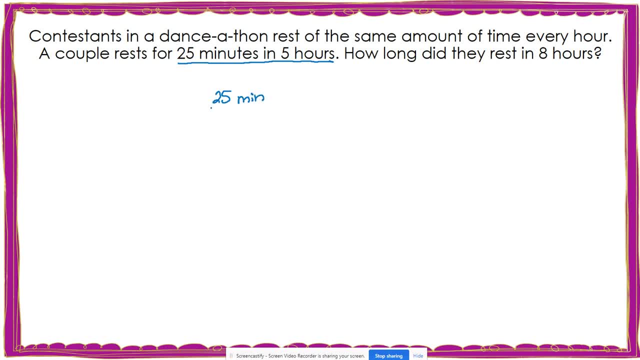 so the couple rests for 25 minutes in five hours. that's my first ratio. now I'm trying to find how long they rested and since rested is in my numerator for my first ratio, I'm going to put that in my numerator for my second ratio and since I don't know it, I'm going to put a variable. what? 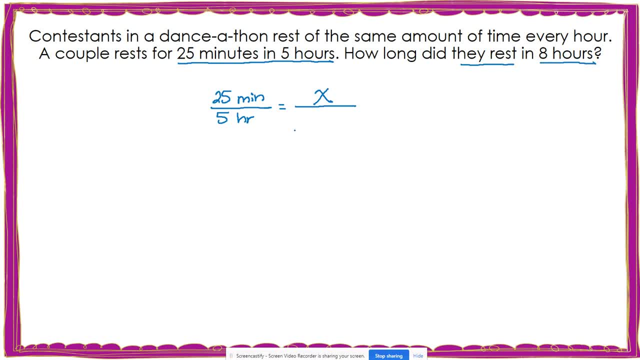 I want to find out is how long they rested if they danced for eight hours. since hours are in my denominator for my first ratio, they're going to be in the denominator for my second ratio. now I can't easily see how I move from 5 to 8, so this is one of those situations where using a using 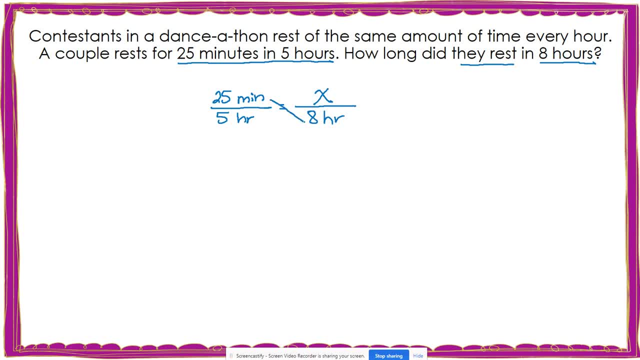 cross multiplication would actually help us. so I would multiply 25 times 8, which would give us 200, and then I would put my equal sign. then I would multiply x times 5, which would give us 5x, and now, to get X by itself, I would divide by 5 on both sides of my equation: 200 divided by 5 is 40. 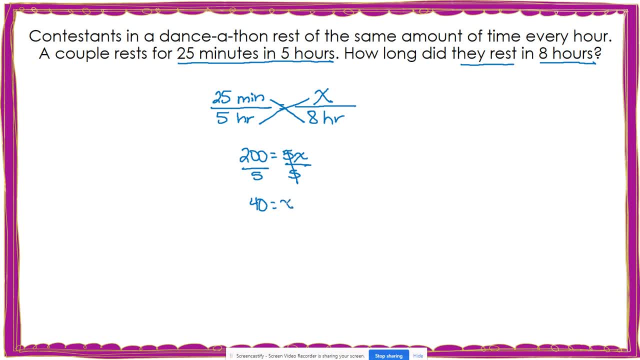 my 5 divided by 5 is 1, and 1x leaves us with just X, so the fives cancel. this means that X equals 40, so the couple rests 40 minutes in 8 hours. next, I see that Francis gets six paychecks in 12 weeks. how many paychecks does she get in one year? 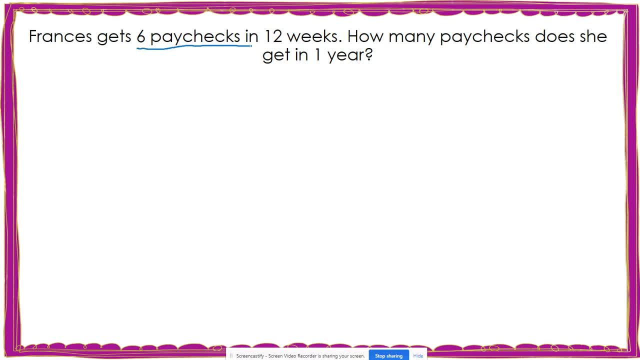 well, let's start with what we know first. we know that she gets six checks in 12 weeks. the question wants to know how many paychecks does she get in one year? the problem is when I compare my first ratio, my first ratio is 53 times shy ofIf I am asked to convert my two second ratio shooting number to weeks. 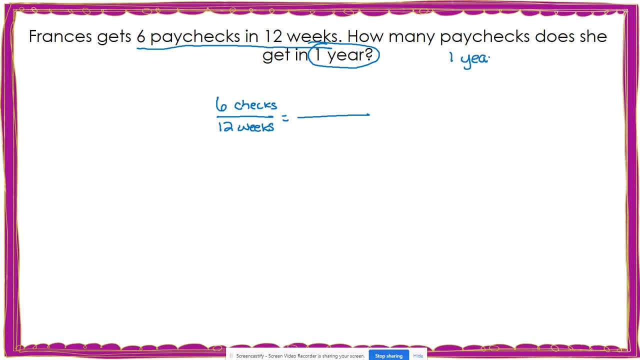 on the state of 1st ratio may be constantly changing, so we immediately we put my first ratio into my second ratio. when I am taking my second ratio shot, I'm also put into my second ratio because I'm seeing that there's now plus, plus, plus, plus, plus over there. so I need to convert. 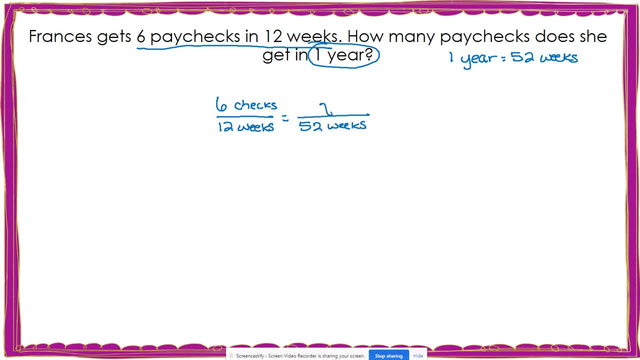 my second ratio, how many paychecks Francis gets. So I'm going to put that here. Now I can cross multiply. So I'll multiply six times 52,, which gives me 312.. Then I put my equal sign. I multiply X times 12,, which is 12 X. 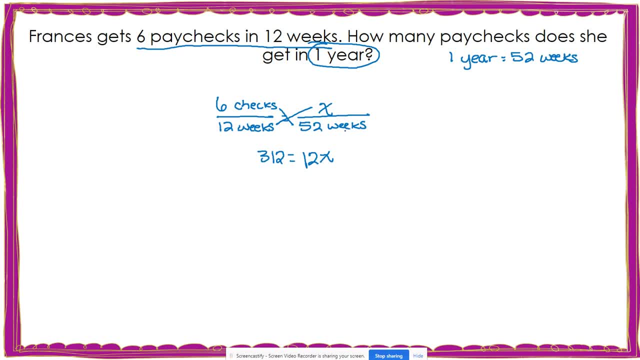 Now I'm just going to get X by itself by dividing by 12 on both sides of my equation. 312 divided by 12 is 26.. My 12 divided by 12 is one, which leaves me with one X or just X. 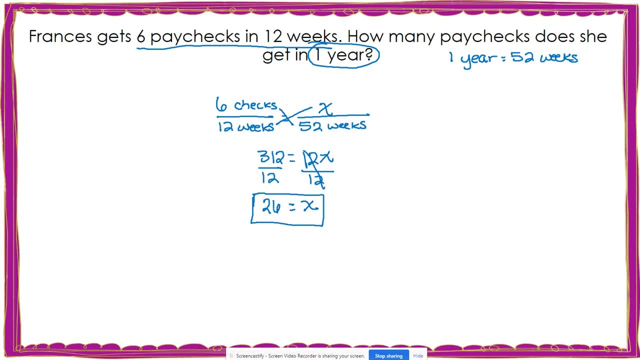 This means that Francis gets six paychecks in 12 weeks. That means that he gets 26 paychecks in one year, or 52 weeks In a repeating musical pattern. there are 56 beats in seven measures. How many measures are there in 104 beats? 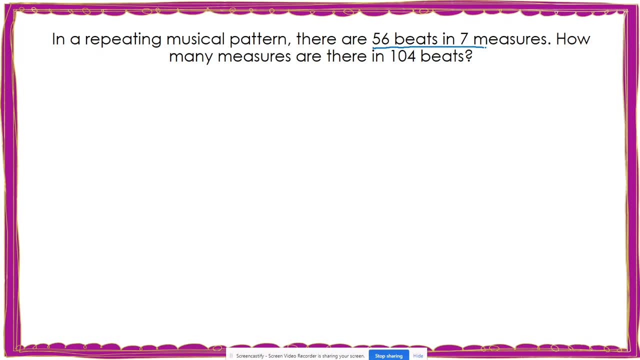 So let's start with what we know. We know that there are 56 beats in seven measures, So we can make a ratio out of that to show 56 beats for every seven measures. Now I want to know how many measures. So in this case, I do not know how many measures. 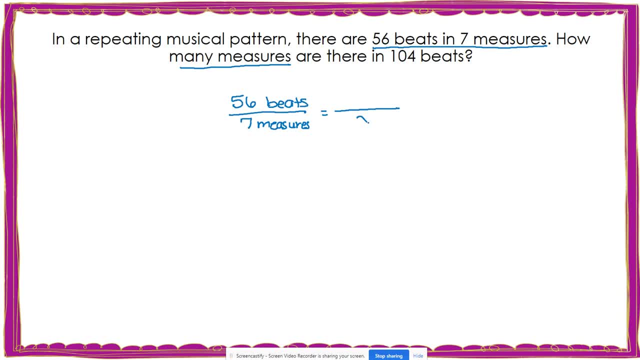 since measures are in my denominator over here, I'm going to put a variable measures in my denominator on my second ratio This time. I know that there are 104 beats, so I'm putting 104 beats in the numerator and now I can cross. 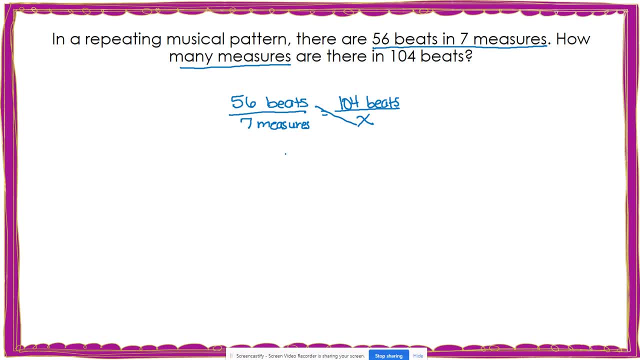 multiply. I'm going to multiply 56 times X, which would give me 56 X, and then I put my equal sign. Then I'm going to multiply 104 times 7, which would give me 728.. Now to get X by itself, I'm going to divide by 56 on both sides. 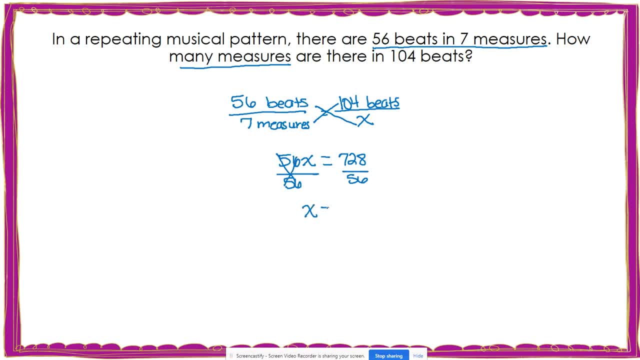 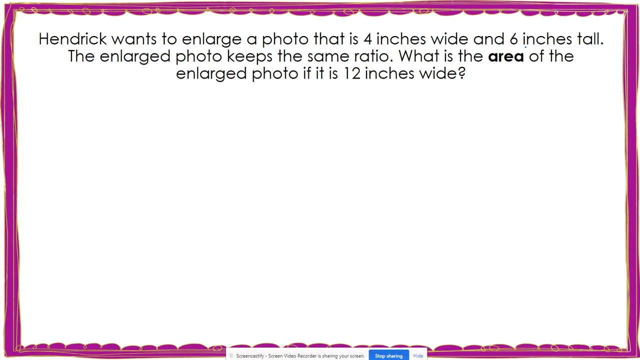 My 56 will cancel, which will leave me with X equals, and then 728 divided by 56 is 13.. This means that there are 13 measures in 104 beats. Hendrik wants to enlarge a photo that is 4 inches wide and 6 inches tall. The 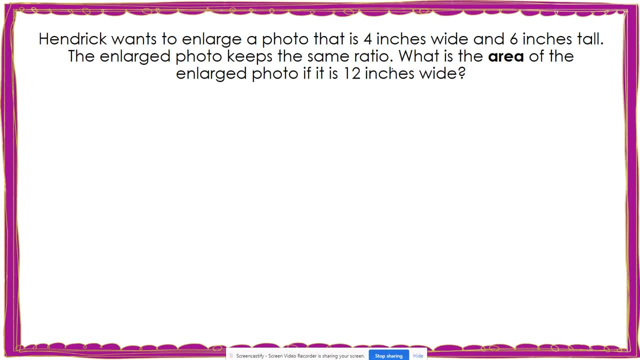 enlarged photo keeps the same ratio. What is the area of the enlarged photo if it is 12 inches wide? So the photo is enlarging at the same rate. so we're going to start with the original photo. Our original photo was 4 inches wide and 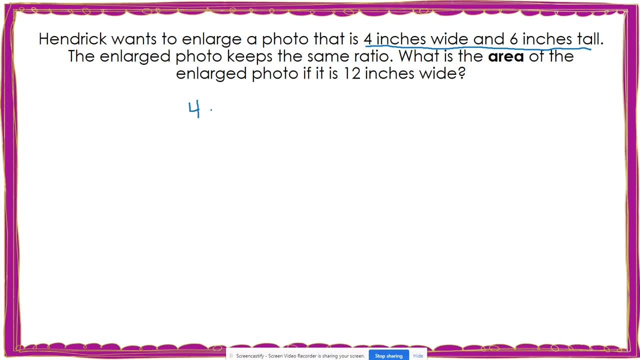 6 inches tall. so that's going to be our first ratio. It's 4 inches wide, 2 inches wide and 3 inches tall. Next, we know that we are looking for an enlargement that makes it 12 inches wide. Since my wide is on my numerator, for my first ratio, width is going to be: 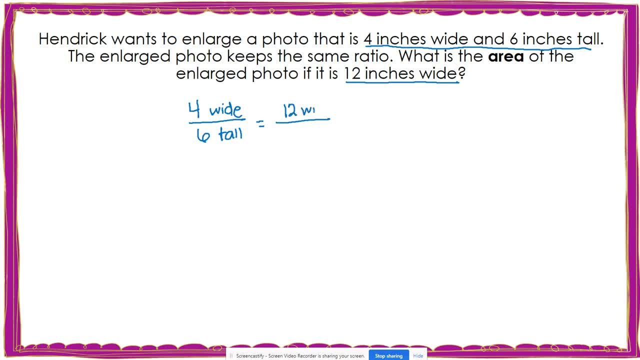 in my numerator for my second ratio. What I don't know is how tall that enlarged photo will be, so I'm going to put a variable to represent that. Now for this one, I can see that if I move from 4 to 12, I 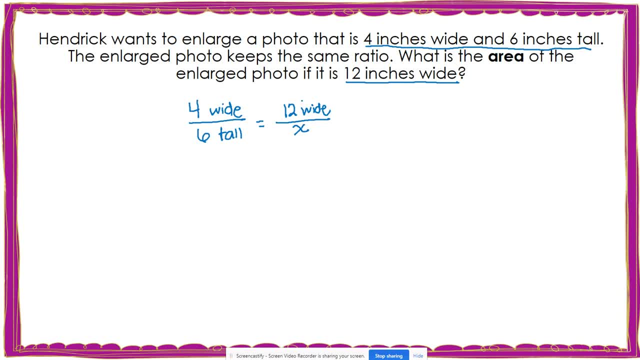 can pretty easily see that I can multiply 4 times 3 to get to 12, which means I would also multiply 6 times 3 to get to X. So I can see that X would be 18. but if you can't see that, or if you just prefer using a cross, multiplying to,